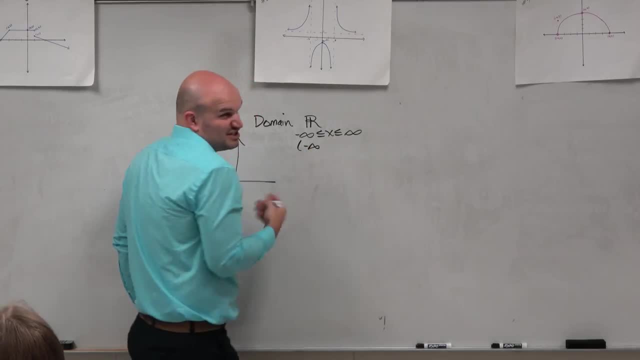 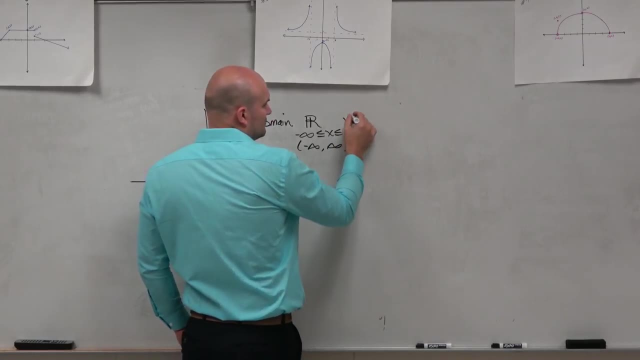 We could also say, just we could represent this as negative infinity, because there really is no place, it's going to stop, right? So the reason why I bring this up: that's fine Mathematically correct. That's fine Mathematically correct. 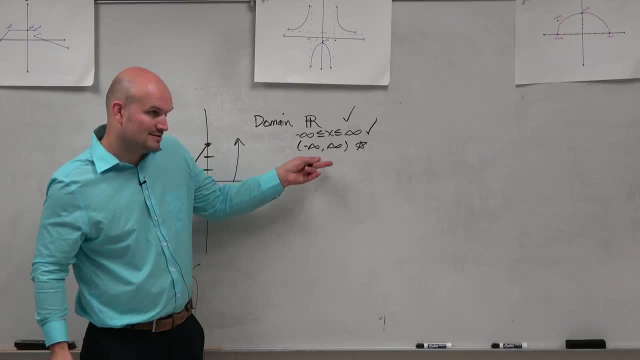 Guess what's going to show up on a multiple choice way Test. This is what I'll be expecting. So, on a free response, if you represent all three of those ways, I'm not going to mark you wrong. That's perfectly fine. 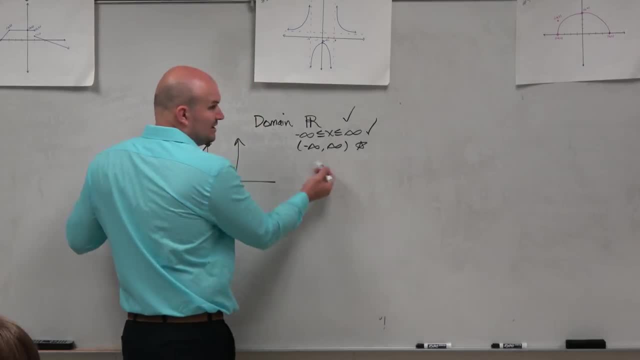 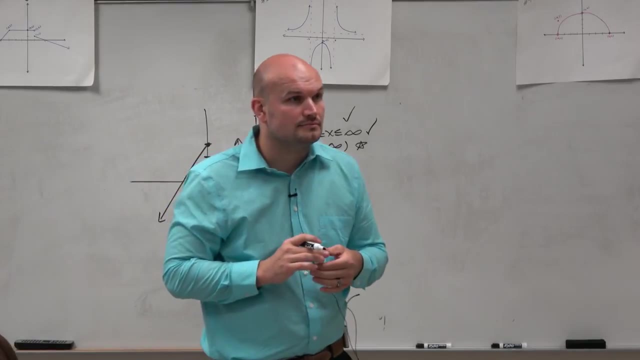 If you prefer one method or the other, that's cool, All right, All right, Cool. However, when looking at multiple choice, I want you guys to get familiar with this, because that is what you will see. Yes, Don't drag this like. 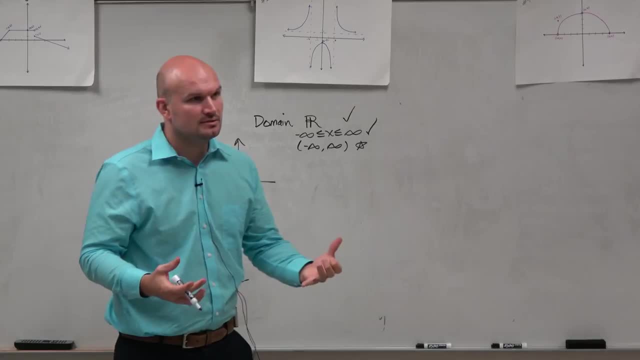 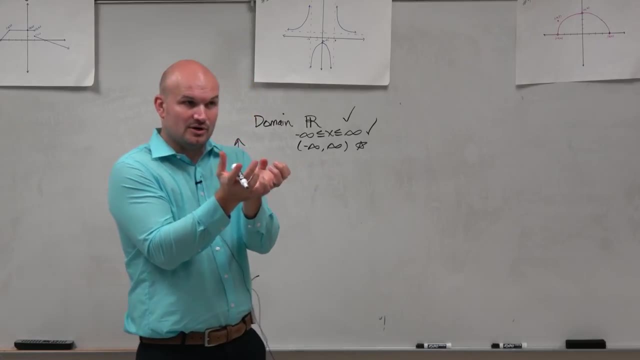 Correct. And so since infinity is actually not a number, you can't grab and say you have infinity of something right? So since infinity is not actually a tangible number that you can actually obtain, that's why it's going to be using parentheses. 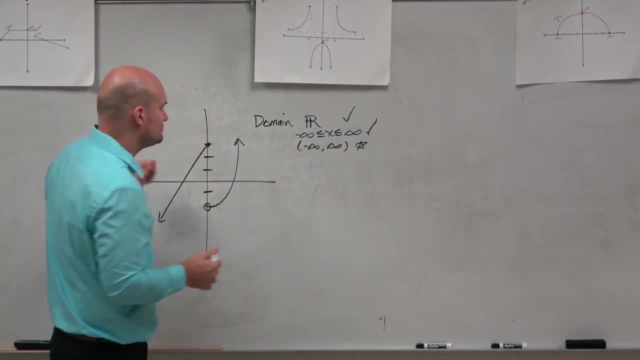 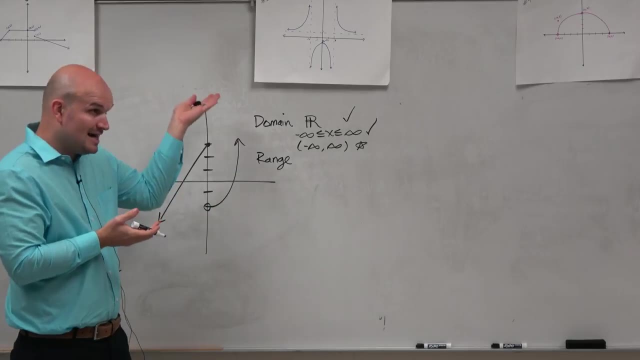 But yes, we will get into that parentheses kind of component. So the range: It's basically asking us how low is this graph going to go and how high is it going. So the range is talking about the y values instead of the x values. 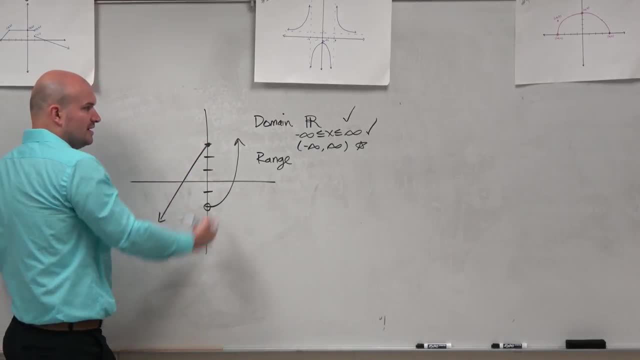 as we did for domain. Well, this one's fairly simple. We're going down to negative infinity and then up to infinity. So, again, this is going to be the same thing. The next one is going to be increasing, decreasing. 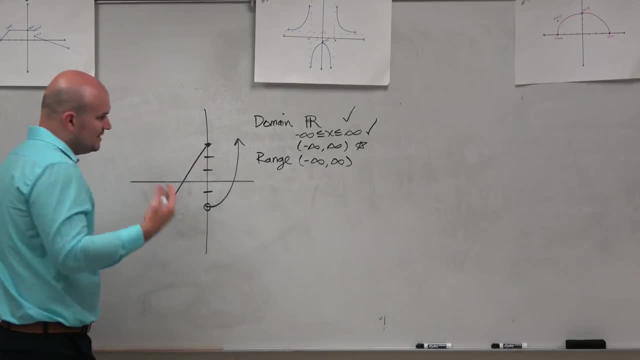 and constant. So when we're looking at increasing, decreasing constant, this is what kind of got to those other things. This is what kind of got to those other students. all right, We're looking at this. You can see that the graph is like when 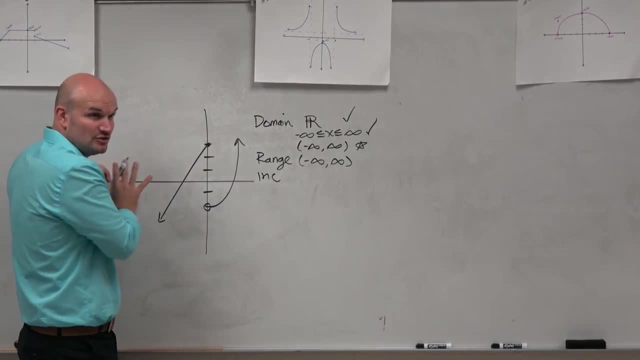 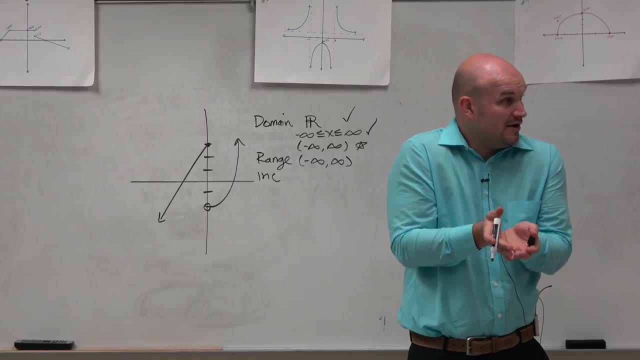 we're reading increasing, decreasing, constant. we're reading the graph from left to right. So, just like a book, we're going to read this graph from left to right And basically we're saying, is the graph going up, is it going down or is it remaining the same? 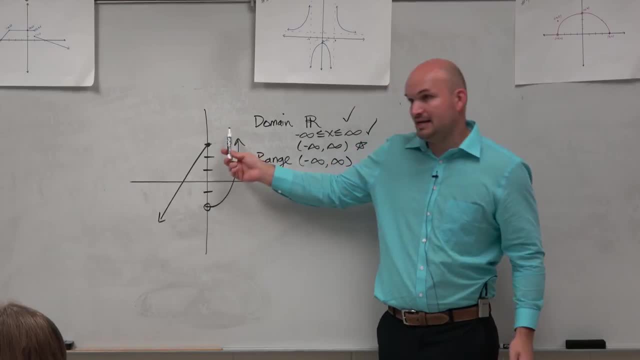 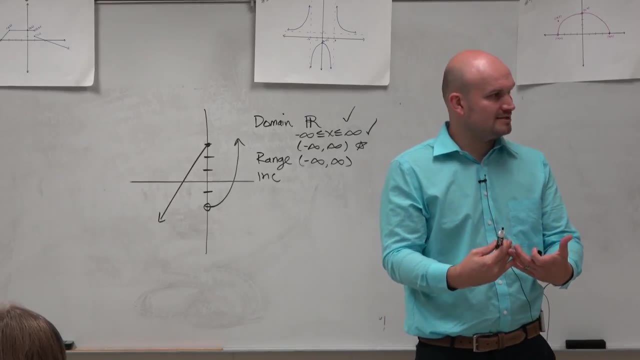 And I think everybody would agree with me. from here to here the graph is going up correct. But again, we've got to be consistent with how we're going to reframe that If we want to make sure that we communicate to everybody what 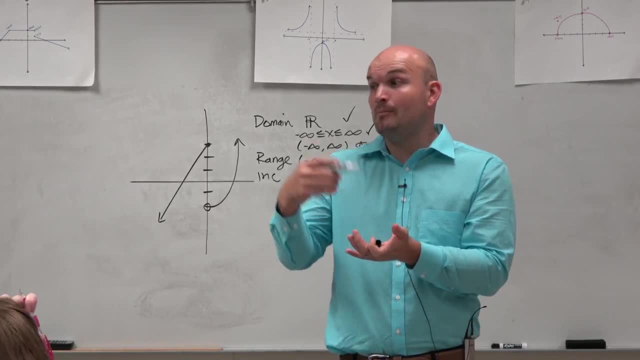 exactly is happening at the end, or exactly what we could say. we could say how much it's going up, or we could say when it's going up. Would you guys agree? You could say it's going up from like 0 to 10,. 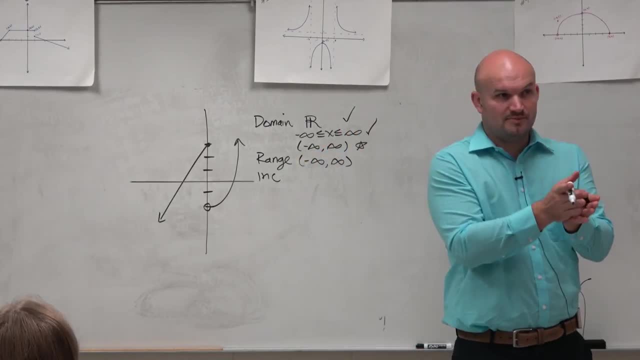 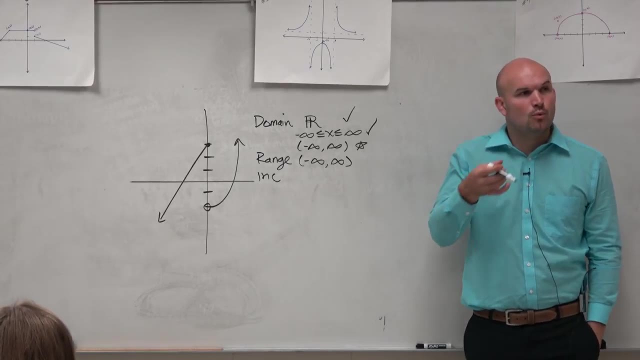 or you could say it's going up from this point to this point. Yes, it's kind of like time versus quantity, right? So the way that we describe increasing, decreasing intervals is when We're not discussing how high or how low, it's going up or down. 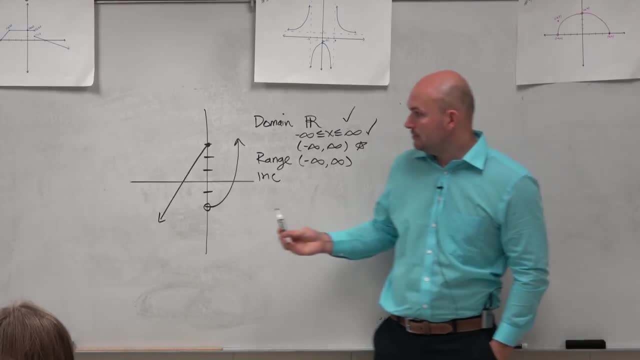 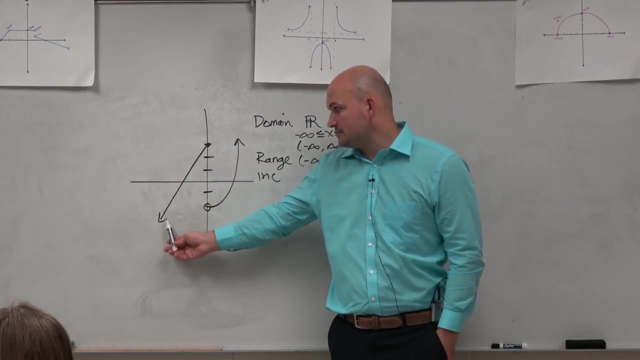 We're just discussing. We're just discussing when it's going up or down. So we can say here, when it's well as far left as we can go, as long as we're moving to the right, this graph is going up. 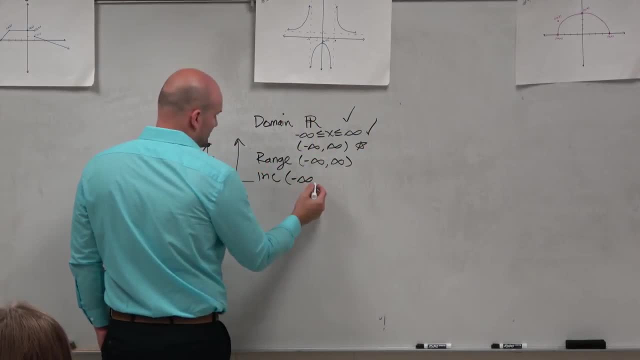 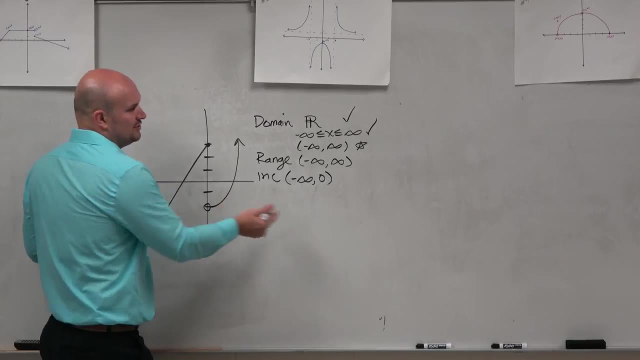 So it's increasing interval from negative infinity to 0. Now technically you could use a bracket here. I avoid using brackets when I'm talking about increasing, decreasing intervals Because technically at the point 0, it's kind of stopped. 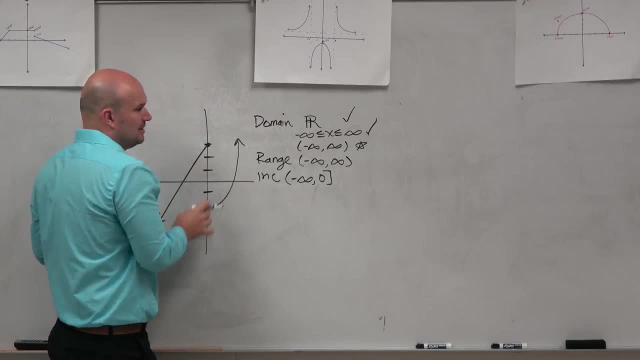 It's not really actually increasing at that value. So therefore, when I'm talking about domain and range, we talk about included, excluded values. But for increasing, decreasing I'm just going to use parentheses at all times. Then as I go from 4, it jumps to here: 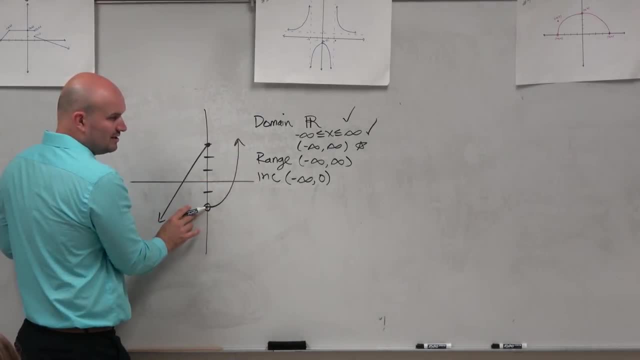 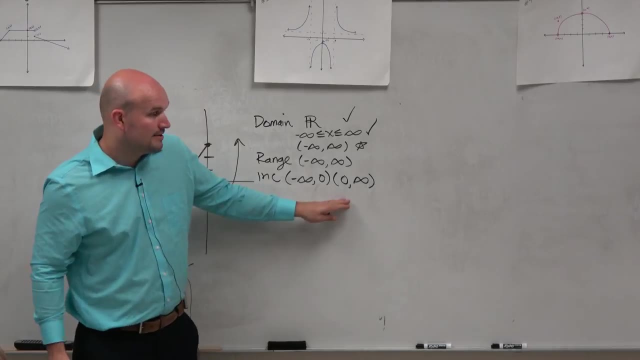 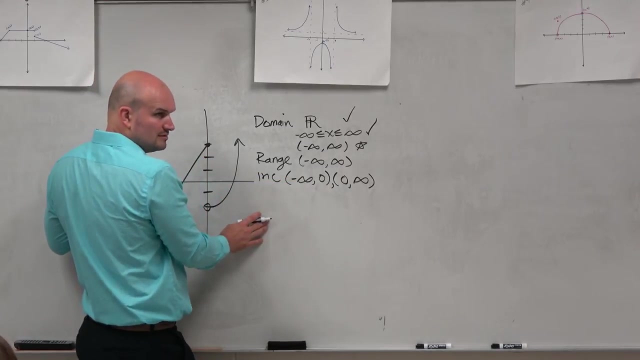 And you can see the graph is again increasing from 0.. And then it's going to continue increasing to infinity. This is perfectly fine, But some students get confused with this and this Like: should we use a comma that connects them? Another way that we will write this and you'll see more often. 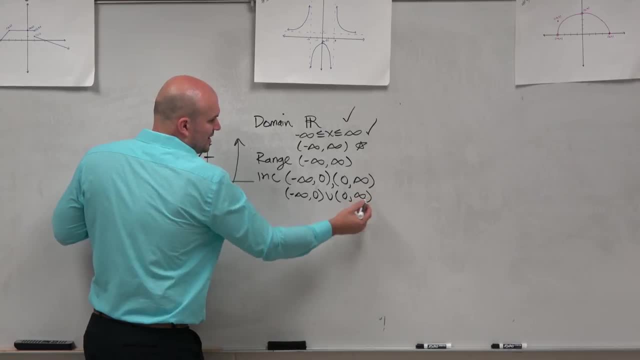 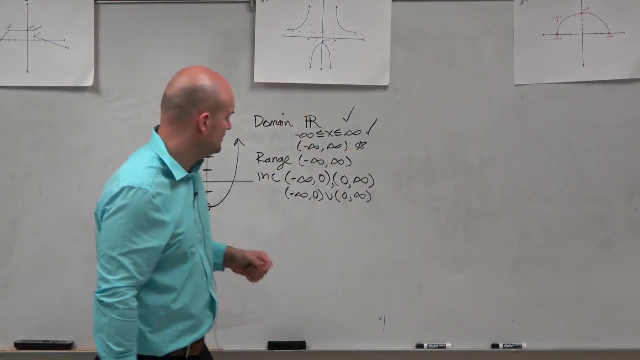 is what we do with the union symbol And if you guys remember, in maybe Algebra 1 or Pre-Algebra, a union is just a combining of those two intervals. So it's just a way to combine those two intervals. Now, is the graph decreasing or constant at all? 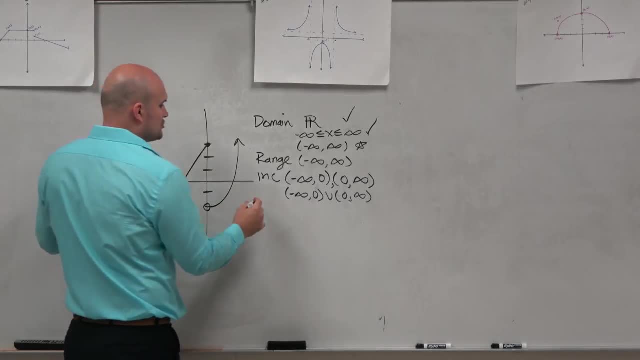 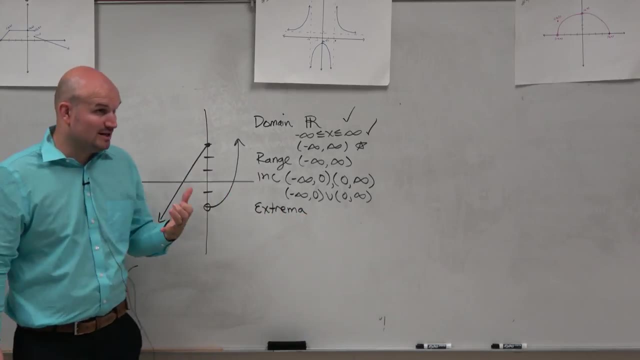 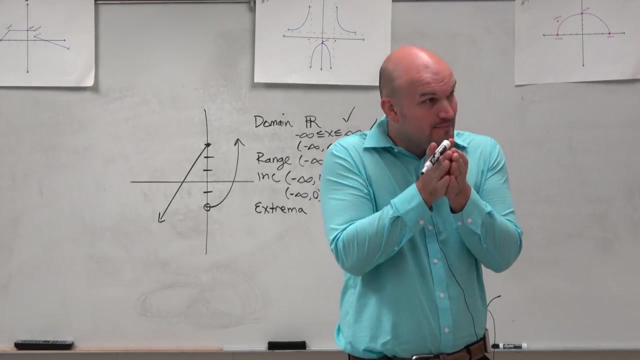 Decreasing or constant? No, We don't need to worry about it. So let's talk about extrema. Extrema is basically saying: where are the maxes and the mins? Where are the maxes and the mins? And actually it's not even that. 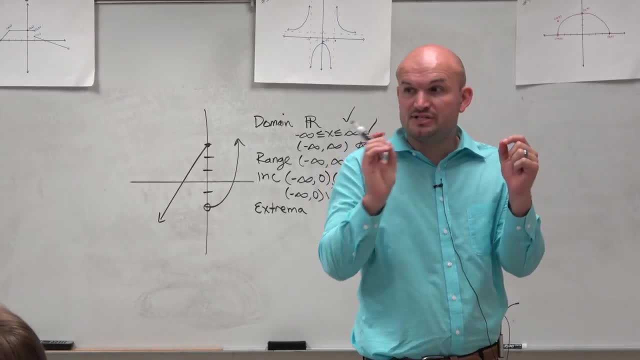 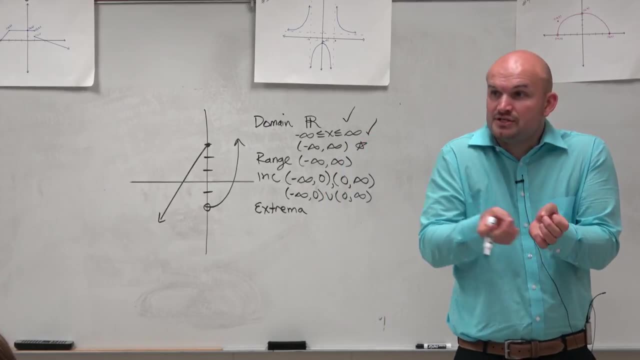 So if it's a max, that means every point to the left and every point to the right is below that value, Correct. And if it's a min, that means every point to the left of that point and every point to the right of that point is above. 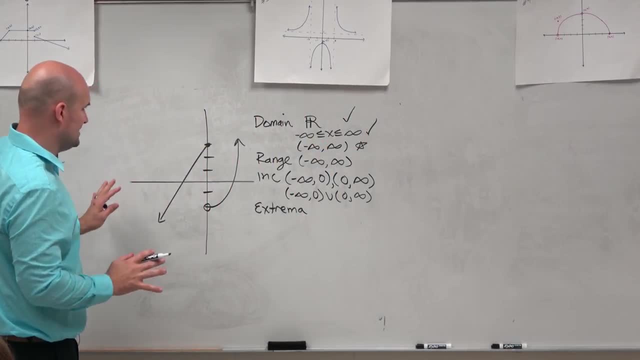 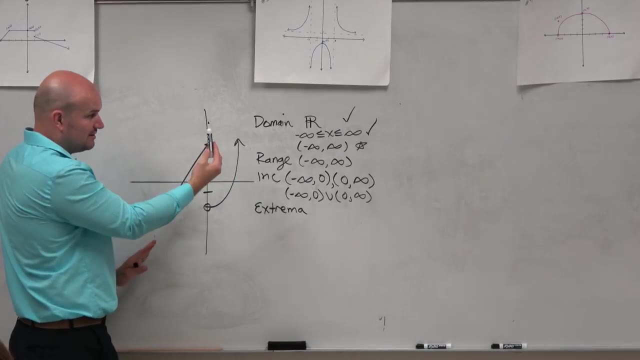 So if we're looking at this, if we want to identify max and mins, well, we notice these arrows kind of mess up. There is no absolute maximum or minimum right. This graph is going to continue without bound. However, if we were to zoom in right there, 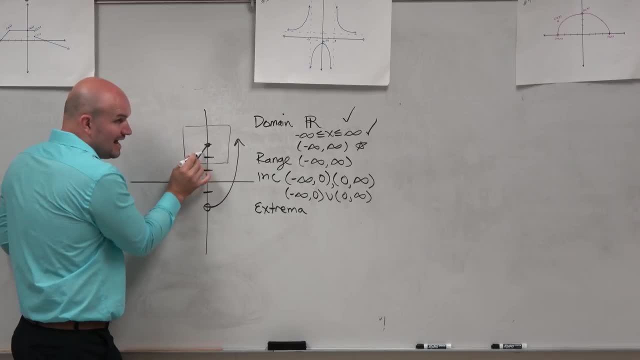 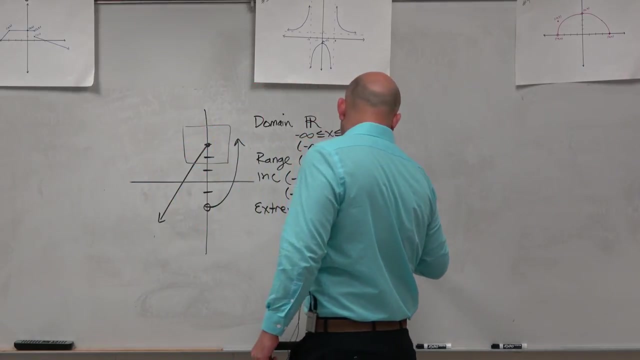 we could say: well, this point right here, anything to the left is above it and anything to the right is above it. Correct, Right. So this is what we call a relative Max. It's not the absolute When we're talking about absolute. 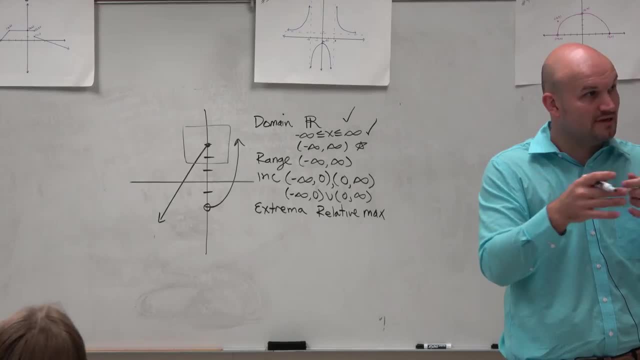 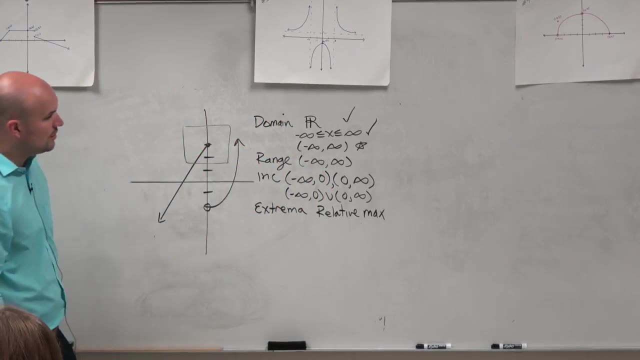 that's talking about the absolute highest point on the graph or lowest point on the graph. When we're talking about relative, that just means within a given snapshot. So this extrema is our relative, That's a relative max. And now there's a couple ways we can do this again. 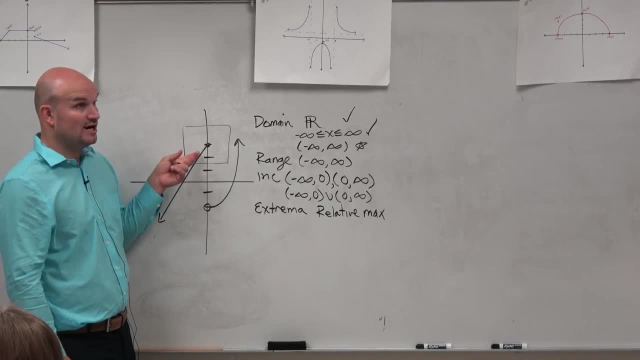 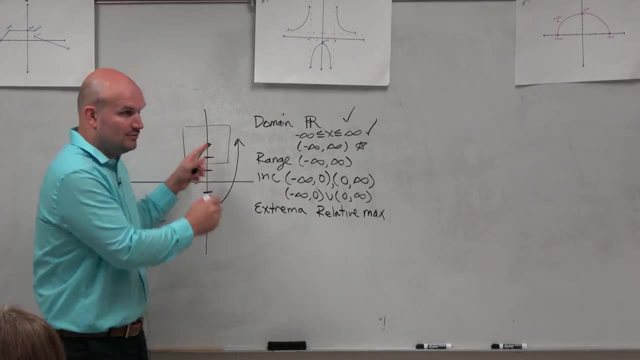 We could define this relative max, where it occurs which you'd be the x-coordinate, or how high is it which would be the y-coordinate. Wouldn't you guys agree? Couldn't we say: there's a relative max at x equals 0,. 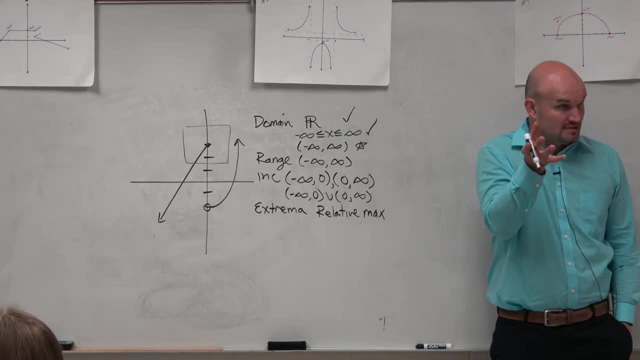 and that would explain to you where that relative max occurs. Yes, Or couldn't you say there is a maximum value? a relative maximum value of y equals 3? You guys see that. So I want you guys to understand that there's a difference of the where or the of. 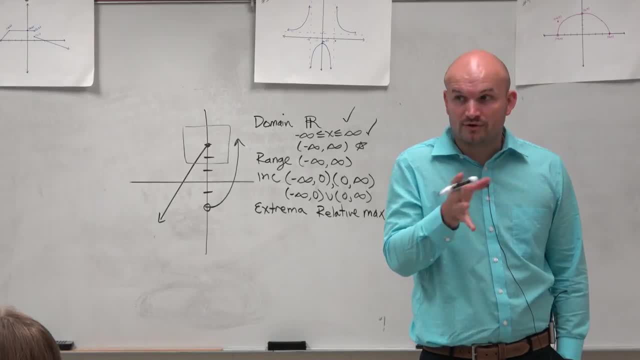 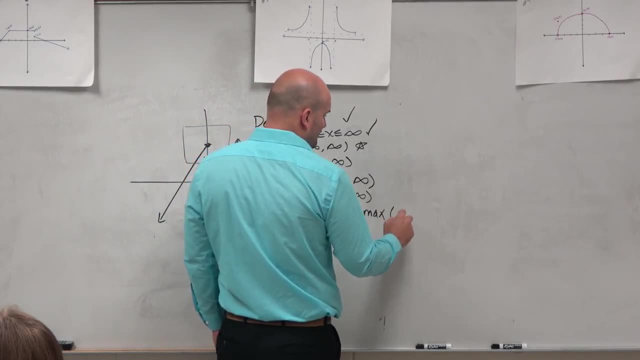 And on tests and quizzes you'll be asked one or the other Like: where does it explain? Now, a lot of times we could just write this: a maximum value of If we wrote 0,, 3, does that take care of the where and the what? 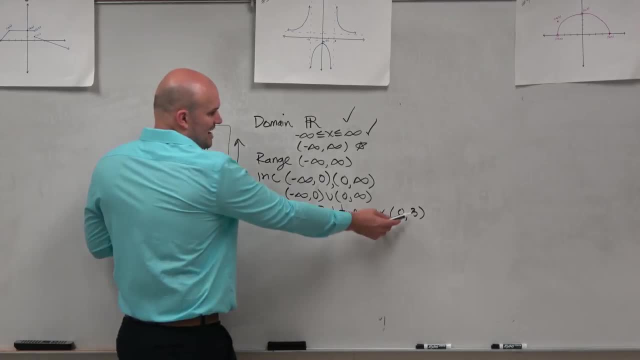 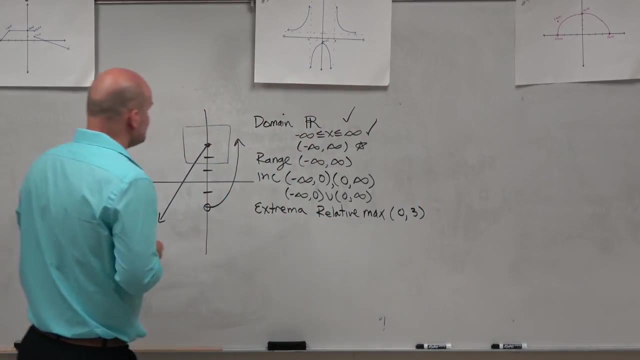 This is saying where it is at: x equals 0, and then what the maximum value is of 3.. But just be aware of the question. Sometimes the question will define other things, But I'll leave this as a coordinate point. Boundness. 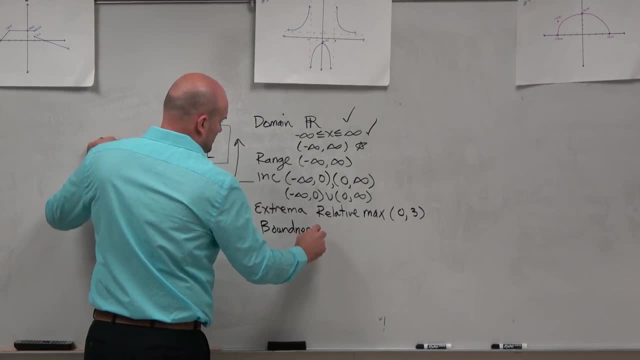 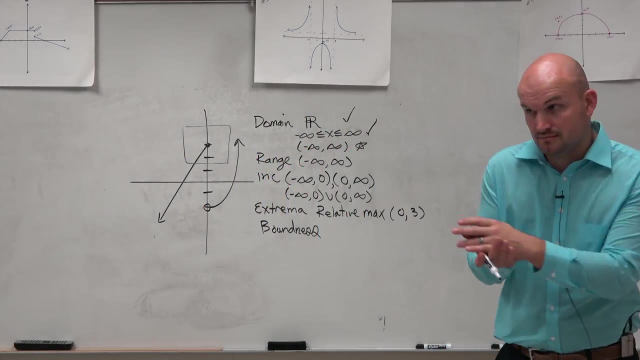 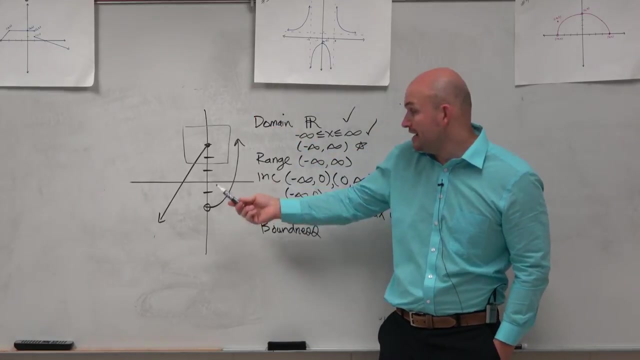 So I kind of actually gave this one away. So the boundness is basically telling you: is the graph restricted? And you guys can see: is this graph restricted? No, It goes without bound up and it goes without bound down. So this is what we call unbounded. 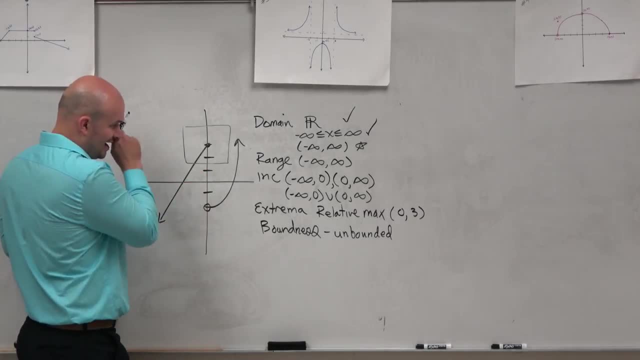 So if there was like, for instance- let's just have for an example- if the graph just looked like this: OK, Is this graph restricted going up? Yes, It has an absolute maximum up there. So this is what we call bounded above. 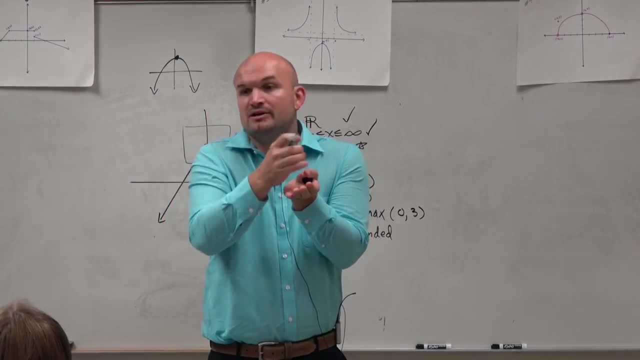 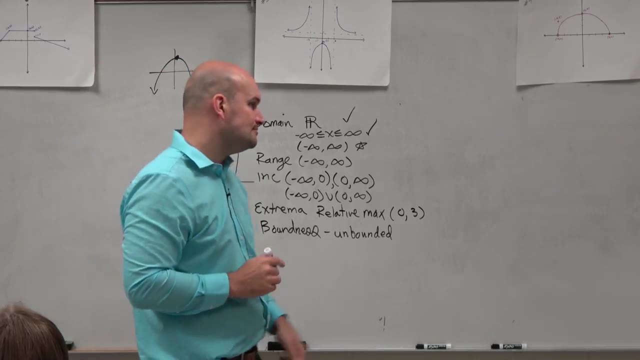 So if there is a restriction, if it only goes so high, then we say it's bounded above, It doesn't go any higher than a given point, And we'll talk more about this as you guys actually get to them. Let's go and get with nBehaviour. 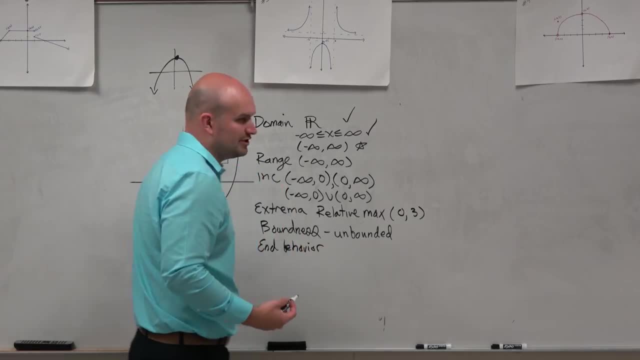 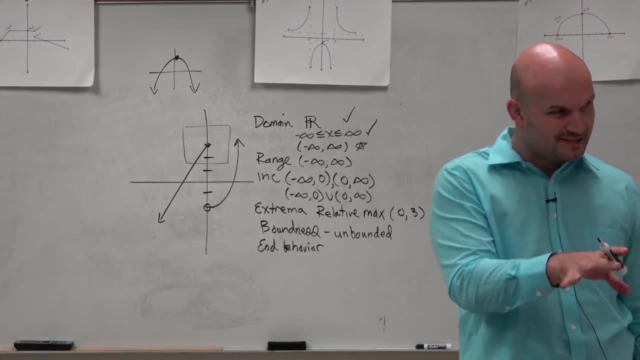 Now nBehaviour is a tricky one. Not really a tricky one as far as understanding, because I think many people can. People can understand nBehaviour, But nBehaviour gets tricky with the notation. So I'm going to keep it simple for today. 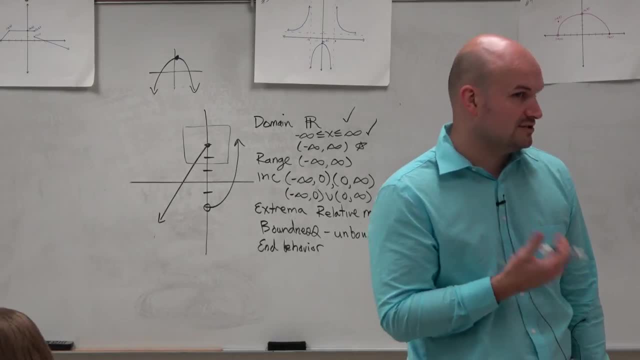 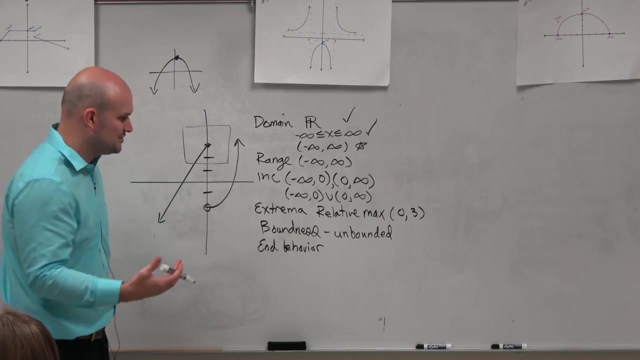 But once we get into next chapter I will introduce more mathematical definitions. So for right now I'll let you guys off easy And we'll just do a very basic notation for nBehaviour, But then we'll get into more mathematical ways. 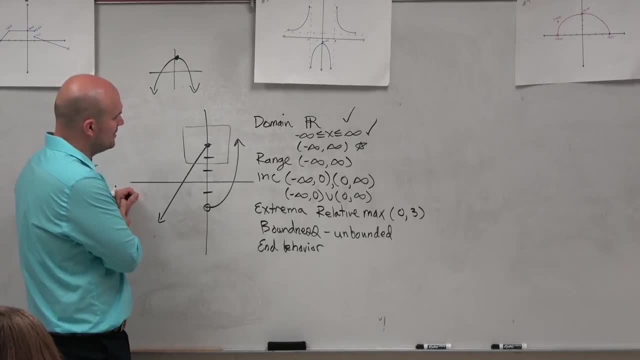 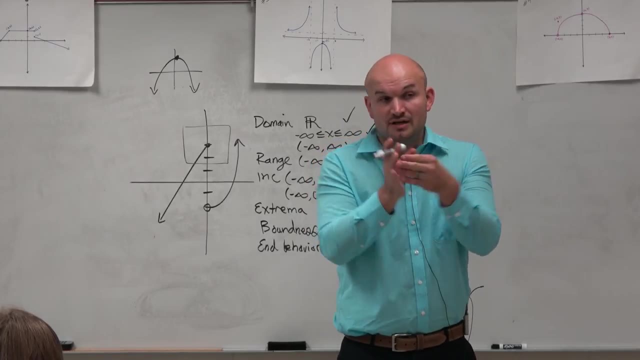 as well as even more calculus ways to describe nBehaviour. So, for right now, though, all the nBehaviour is asking us is: where is the graph going as we go to the right or to the left? So, again, We put back on our reading glasses. 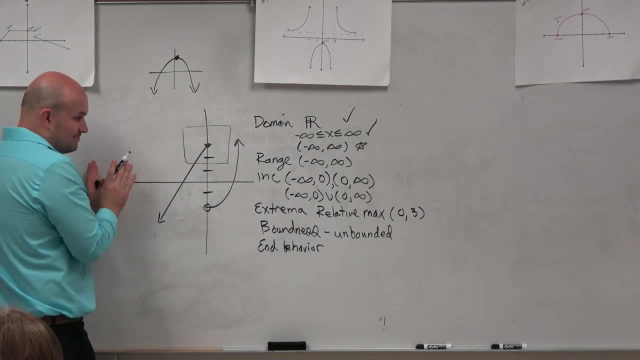 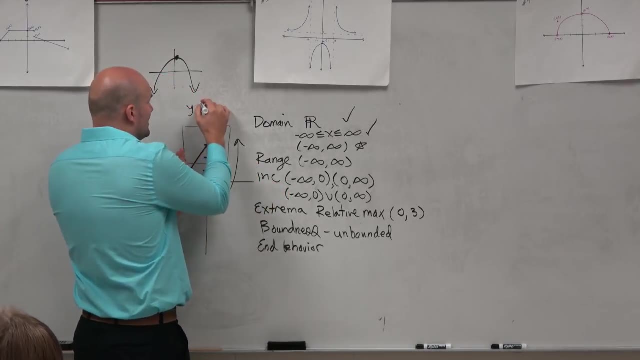 And we say: let's look at the graph As this graph, as I'm moving to the right, as my x values, as my domain is going to the right, where are my y values going? Or y, or f of x, whatever. 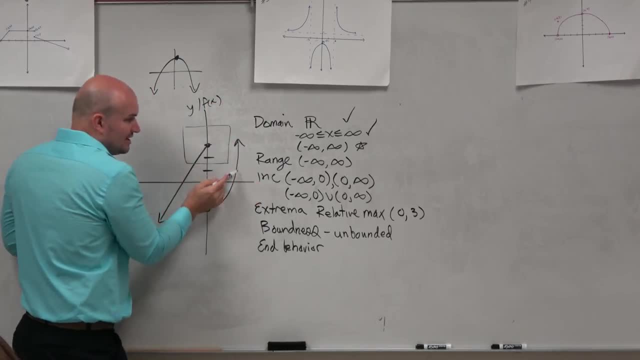 We're talking about an equation or a function. But as I'm going to the right, where is the y values going Up? right, Yes, So you could say it's going up. The one group said it was positive. You could also say it's increasing or it's rising. 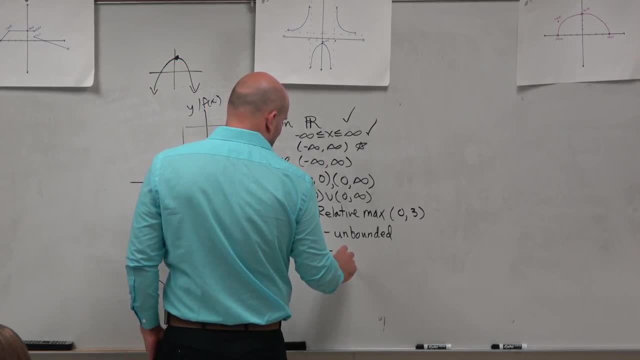 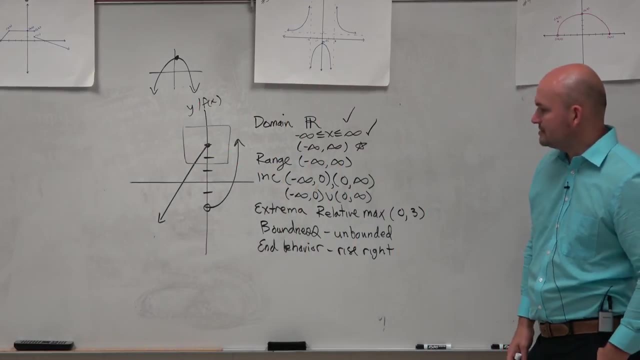 Right. So one way, just a preferred method that I like is it's going to rise to the right And as it goes to the left, as we're moving to the left, the graph is going down. which another way that we say this. 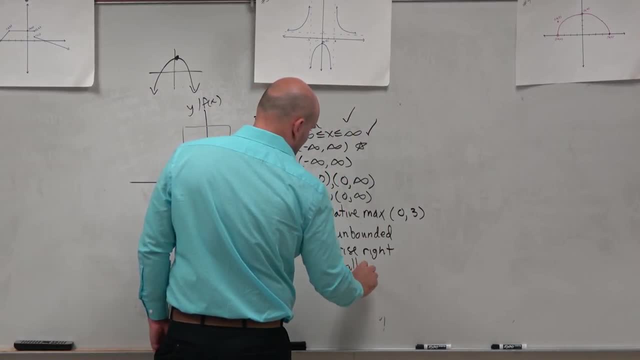 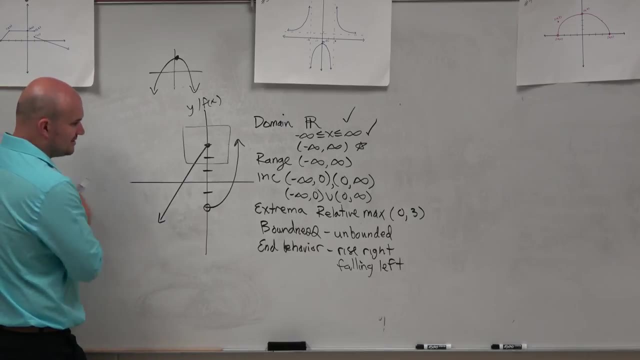 is it's falling, So we could say it's falling left. And then, last but not least, guys- I forgot to mention this, I don't know why I did this, But let's do, let's add some values there. And then the last thing, guys, is the x and y intercepts. 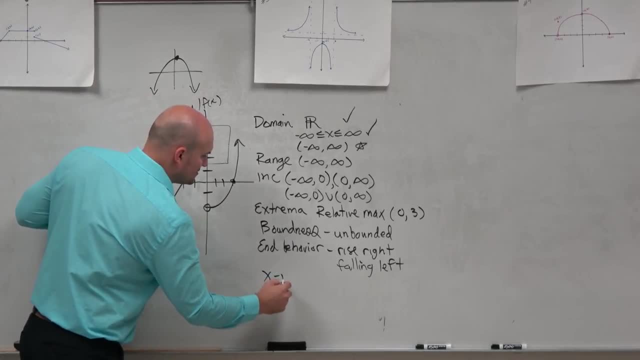 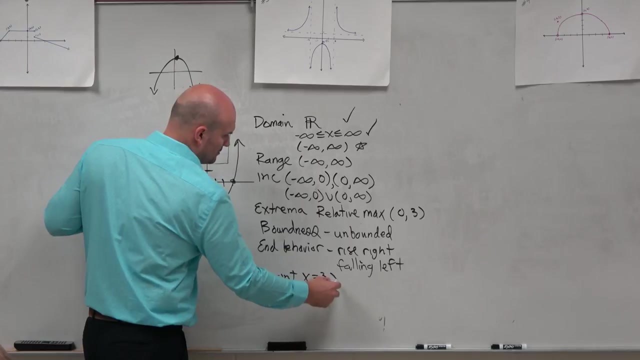 So obviously, guys, the x-intercept is where the graph crosses. OK, And again, you could represent the x-intercept as a value, like x equals 3 and x equals negative 2. Or, depending on the question, you could also: 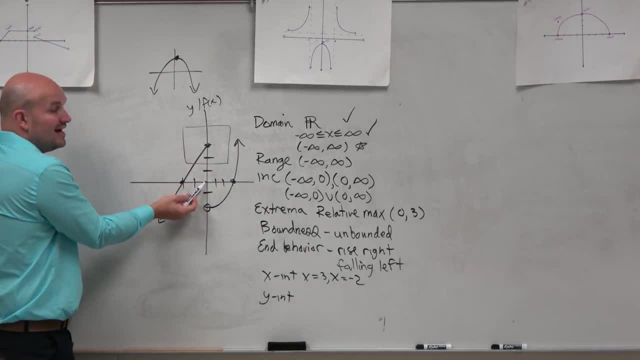 write it as a coordinate point, For instance, giving me the x-value as well as giving me the y-value. And it's important- one thing that's really important- to understand the x-value. what is the y-coordinate of these x-values? 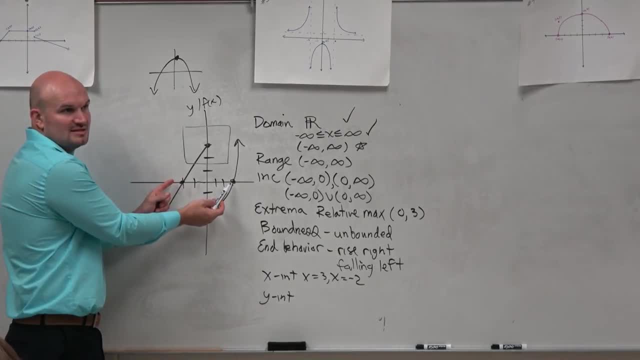 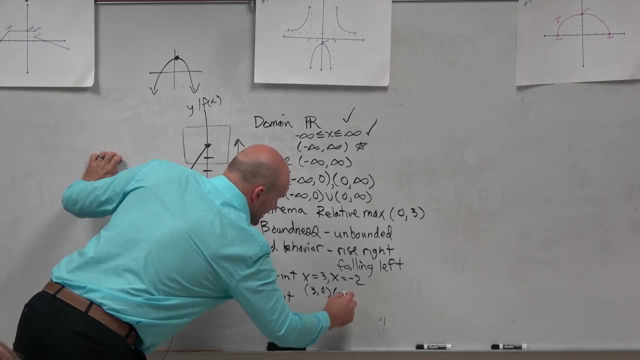 If I wanted to write these as points, what would the y-value be? Starts with the z 0.. So if I wanted to write these as coordinate points, it would be 3 comma 0 and negative 2 comma 0.. 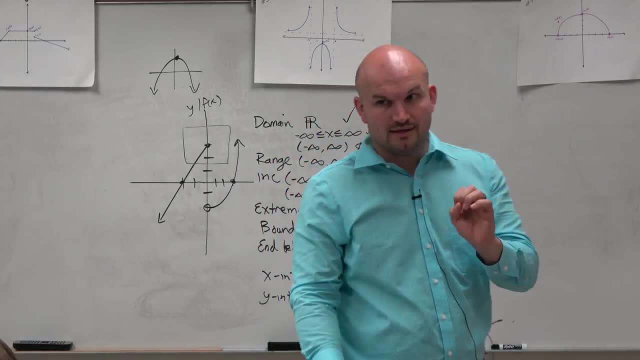 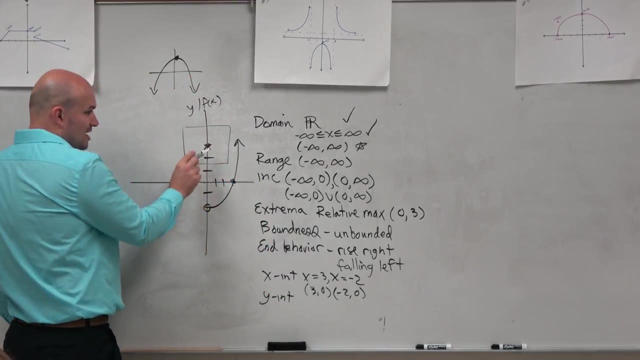 Very, very important for you guys to at least be able to know that and have that done all right. And then the last thing is the y-intercept, which is again where the graph crosses at 1,, 2, 3.. 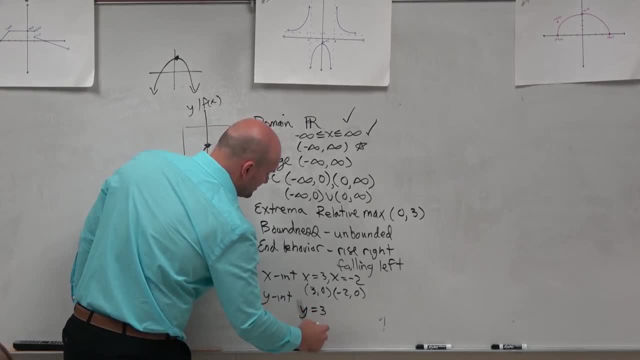 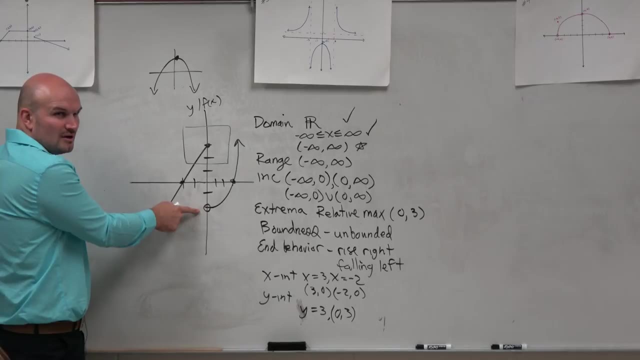 So I'll just write that, as we'd say, y equals 3 or 0 comma 3.. Either one is really acceptable. Is this an x-intercept, though, or a y-intercept? No, because it's a whole right. 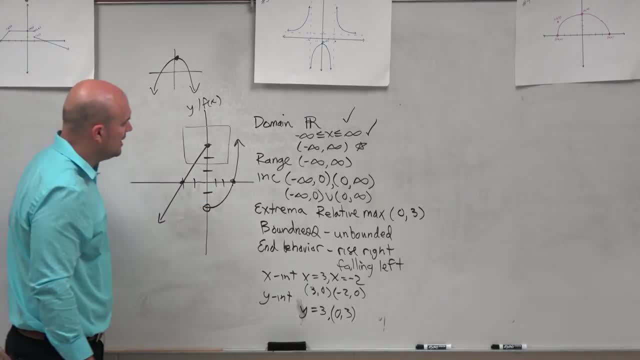 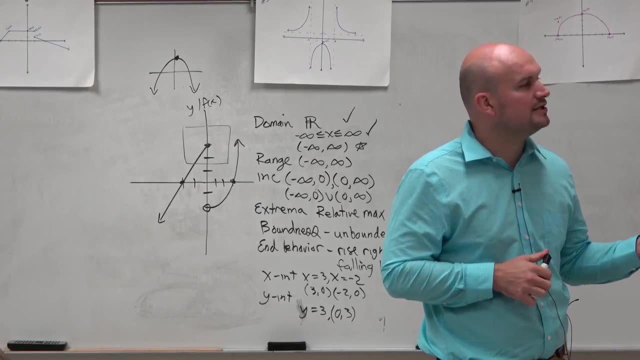 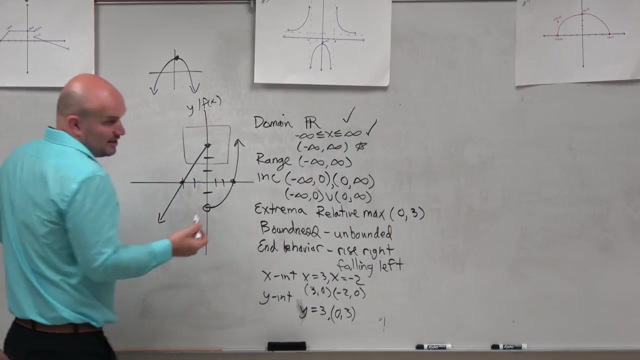 It's undefined at that value. OK, And the last thing I actually forgot to mention is the continuity. So continuity is basically going to be: is the graph continuous or not? And what I mean by continuous is: can you draw? The easiest way to do this is: can you trace the graph? 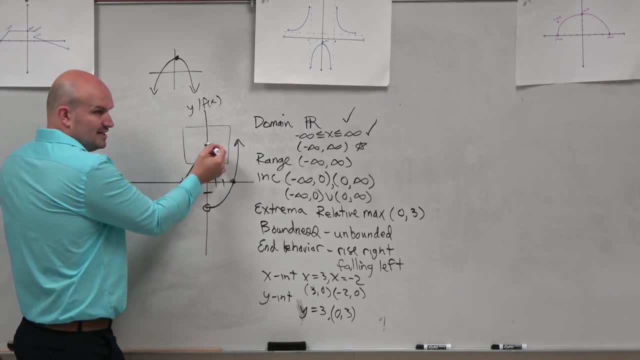 without lifting up your finger or your pencil. And you can see it's pretty obvious that I cannot do that. I have to lift my pencil up, go down over here to continue drawing the graph right. It's kind of like the continuity test. 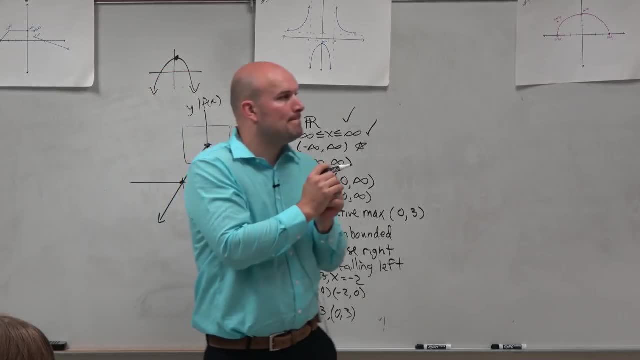 Now, I did mention discontinuities, because I don't want to do that. I don't want to do that. So the idea is to draw on a single graph. We have a bunch of definitions we're going to use, And there actually is some definitions.